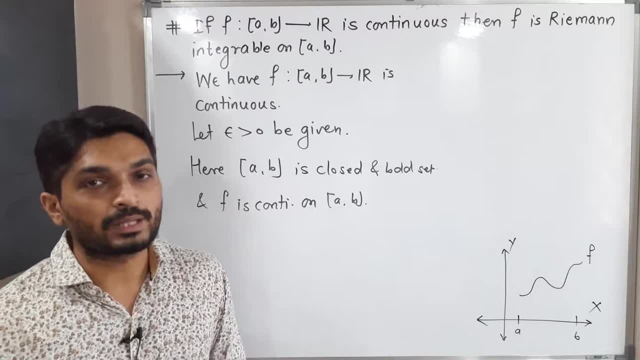 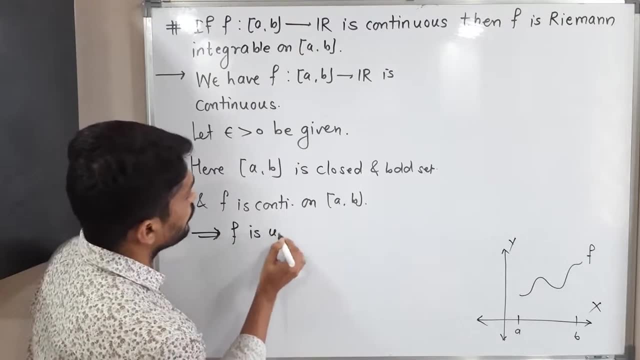 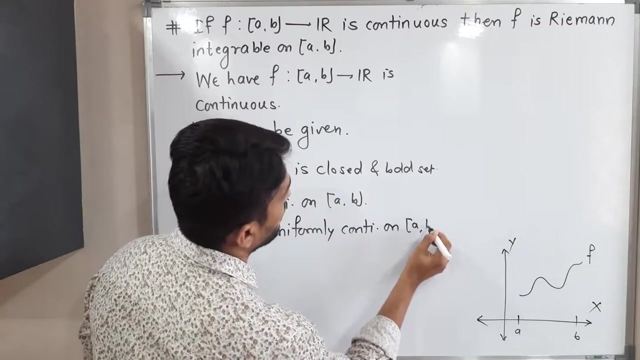 continuous and it is defined on closed and bounded set. Therefore we can say f is also uniformly continuous. Let me mention implies: f is uniformly continuous, uniformly continuous on closed interval a, b. As it is uniformly continuous, definitely we can follow the. 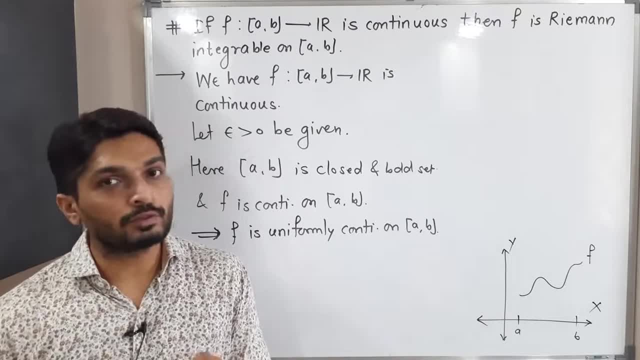 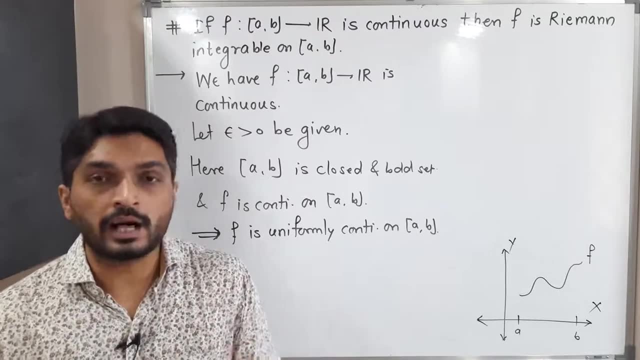 definition of uniform continuity. So definition of uniform continuity says: for given epsilon greater than 0, there exists a delta greater than 0, such that mod x minus y less than delta implies mod f of x minus f of y less than epsilon. So here also we can write: see epsilon. 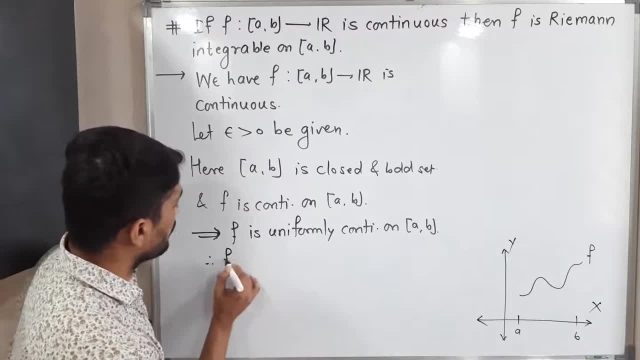 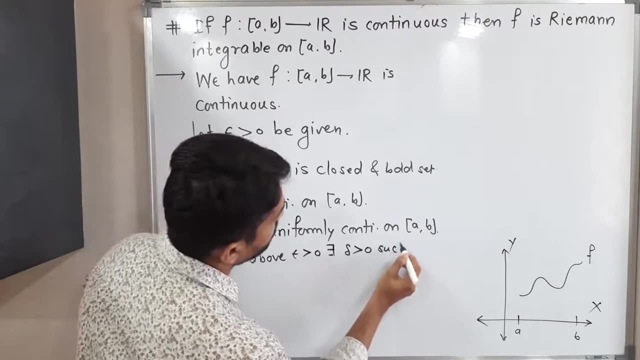 already we have taken. So I will say therefore: for above epsilon, for above epsilon greater than 0. So here also we can write: see epsilon. already we have taken. So I will say therefore: for above epsilon greater than 0, there exists a delta greater than 0, such that mod x minus. 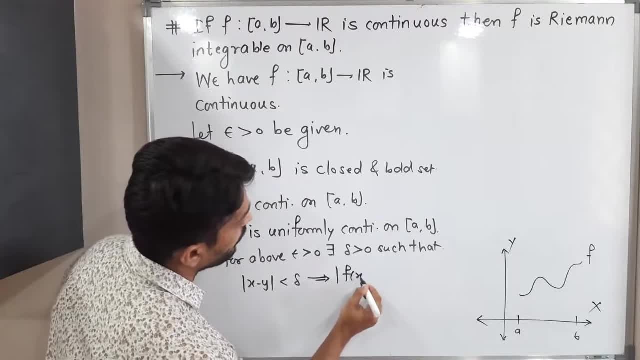 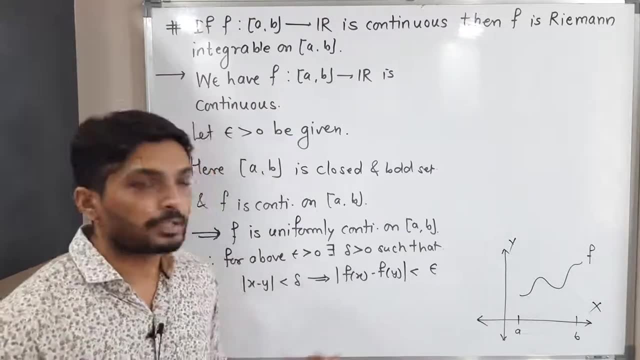 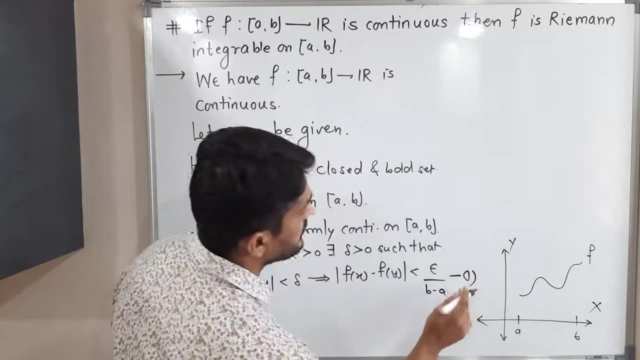 y less than delta implies mod f of x minus f of y less than epsilon. See by definition of uniform continuity. I could write it, but a small adjustment I am going to do: Instead of epsilon I will take epsilon by b minus a. This is adjustment. I am calling it as statement. 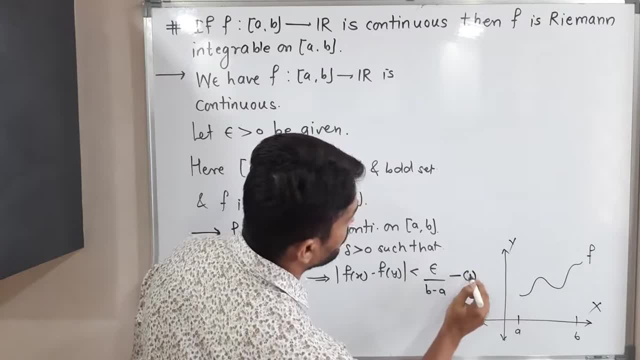 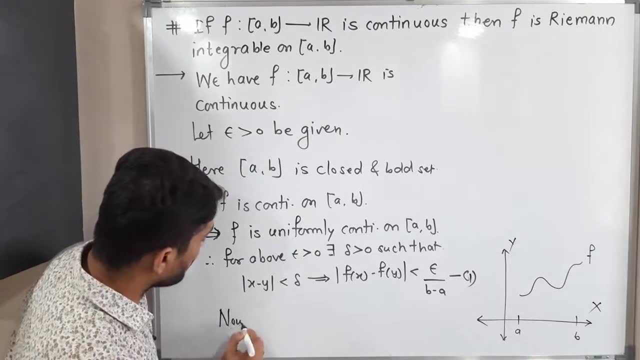 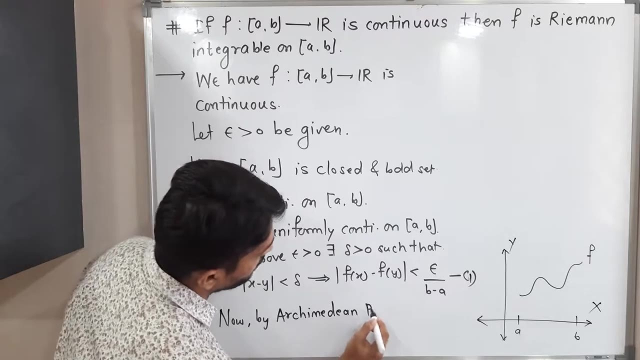 number 1.. It is very important thing we have got. okay, We are going to use it Later. After that, I am going to use Archimedean property. okay, Let me mention Now by Archimedean property. okay, Archimedean property. Do you remember Archimedean property? Okay, Already. 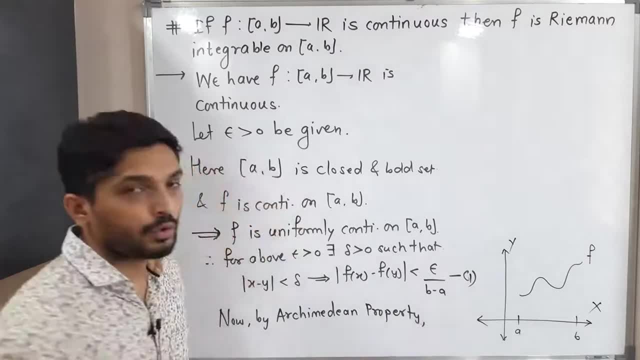 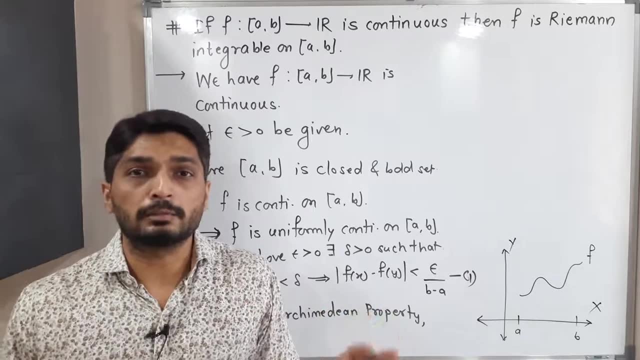 in first year we have already seen: okay, Archimedean property says: for any given real number, definitely you can find natural number greater than that. Okay, So for any real number, you can take x, y, whatever. So definitely we can find a natural number greater than. 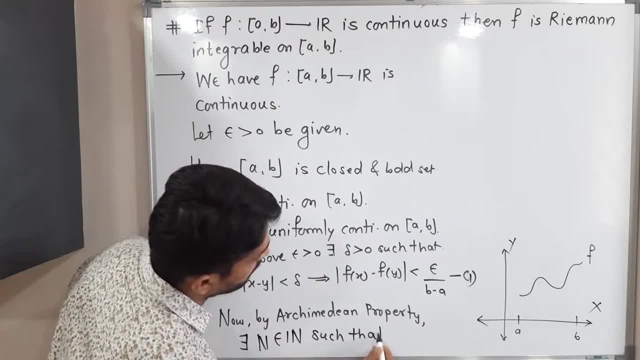 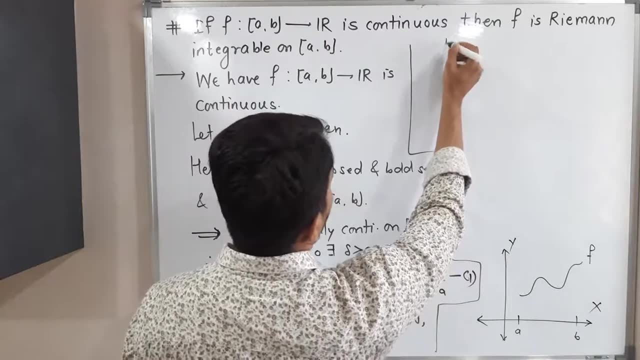 as natural number here, and if we think about b plus b as a minus number here, that is a t here, such that, and if we think about b floor über, über, so that really becomes two, a, several times that one minus two or whatever we have. 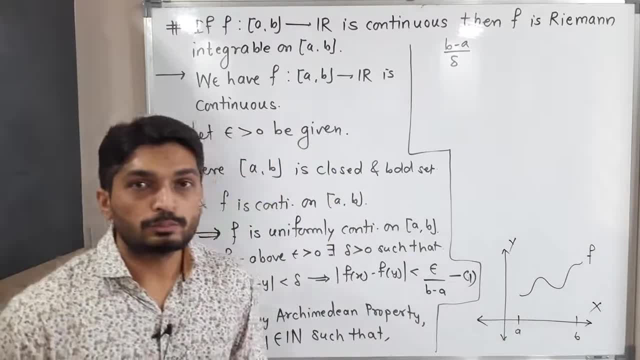 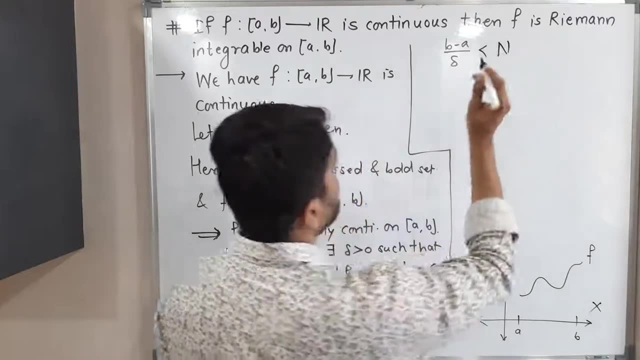 there is a t. right, But relax, If we think about b above b, i times two, i somos a t, then there is a t and there is a t, okay. So when we write about themjang divided by delta, So if you consider this real number, definitely we can find some natural number. 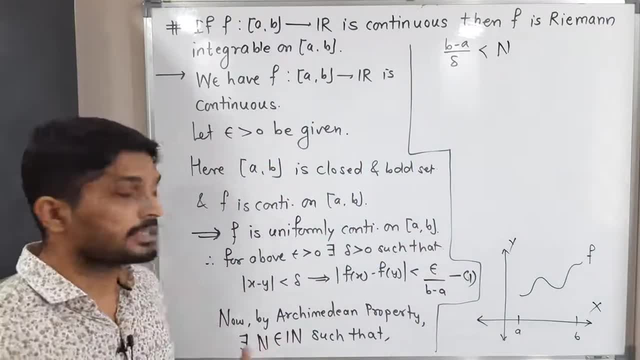 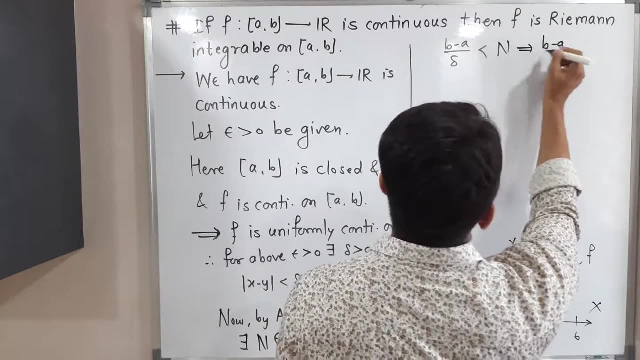 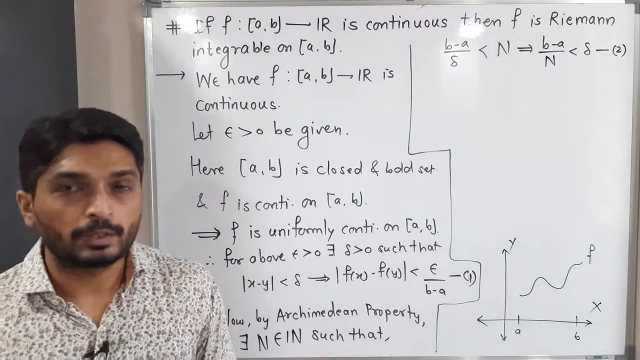 n greater than that We could write just because of this Archimedean property. After that, I will shift n on this side, I will shift delta here, So b minus a by n less than delta. This is inequality number 2. This is also very important thing. So now, what I am going to do, I am going to consider 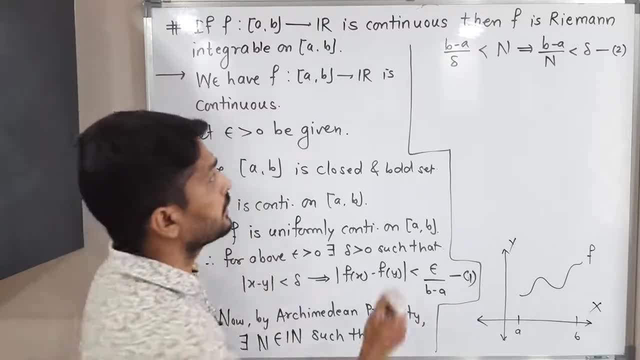 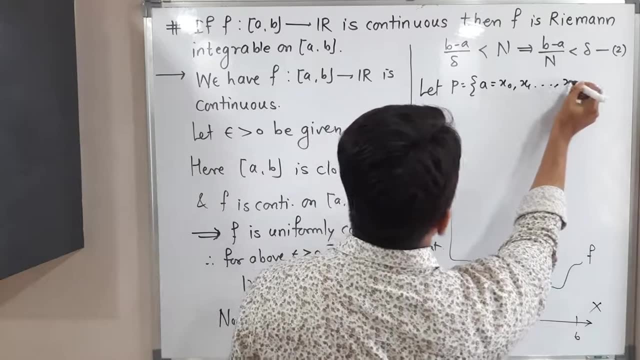 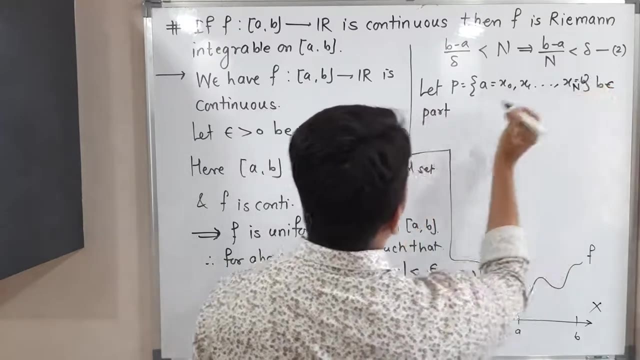 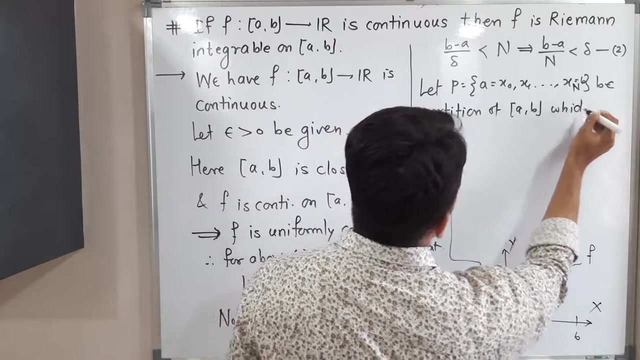 a. partition of this closed interval a- b. Let me mention let. p is equal to a is equal to x, naught, x1, and so on. xn- b partition. Let me mention b partition: xn is equal to b. partition of closed interval a, b which, ok. which divides. ok which divides which divides. 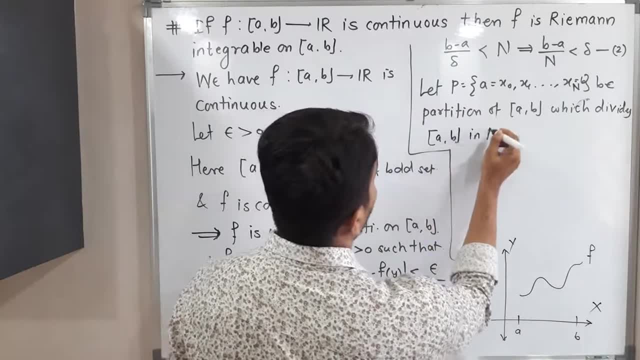 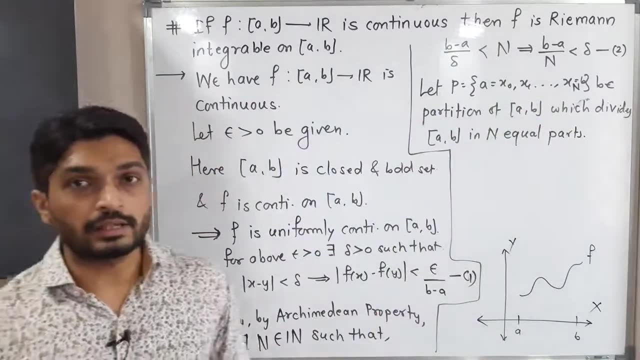 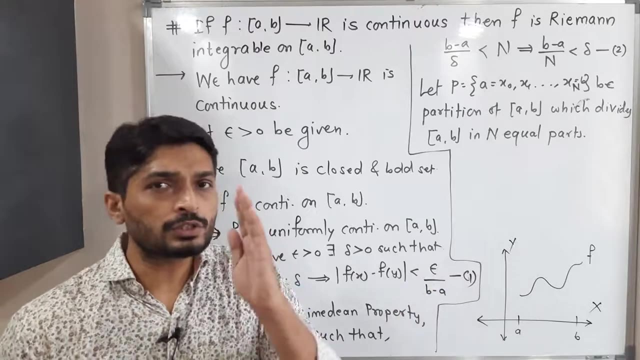 close interval a b, Close interval AB in n equal parts. okay, in n equal parts. So here we have got a natural number, capital N, right? So if you consider natural number, capital N is 100.. So here we consider a partition of close interval AB which divides close interval AB in 100 equal parts, getting 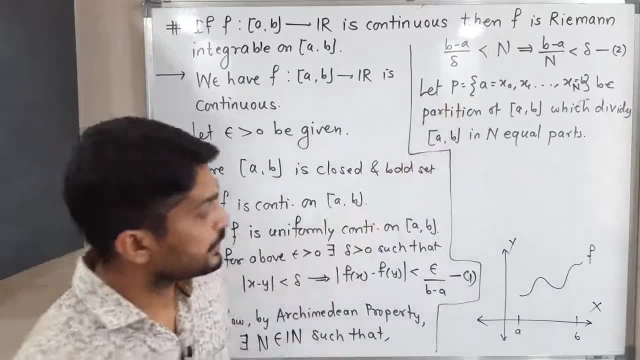 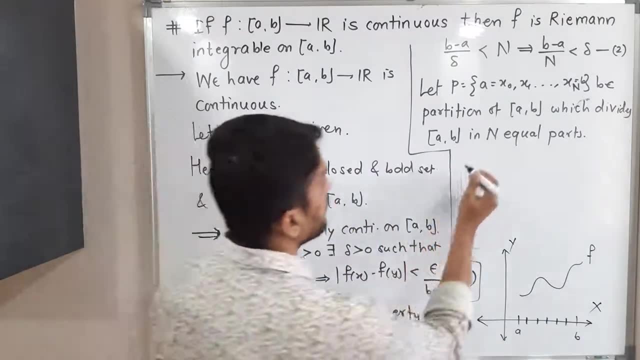 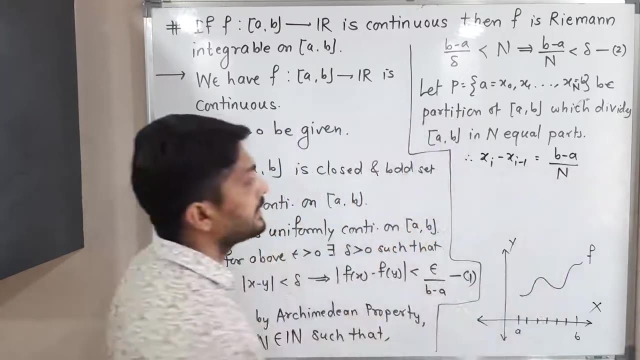 If you consider capital N is 100.. So here we have capital N, So here also we divide AB in capital N equal parts. okay, So therefore length of each subinterval is B minus A upon N. So this denotes the length of each subinterval, right. 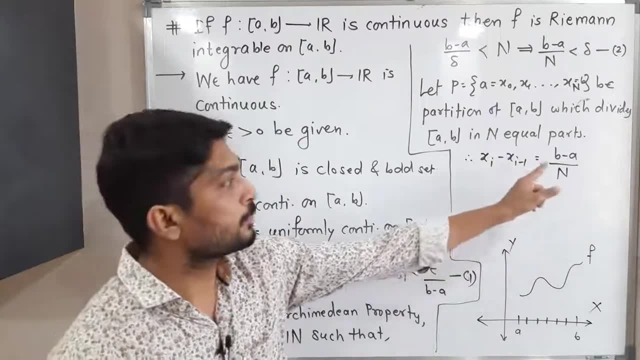 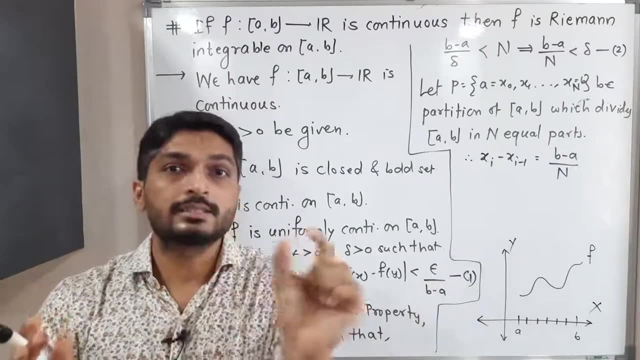 B minus A divided by N. So B minus A means length of that interval, close interval AB. If you divide by N, you will have the length of each subinterval, Since length of each subinterval is 0.. Same equal getting. 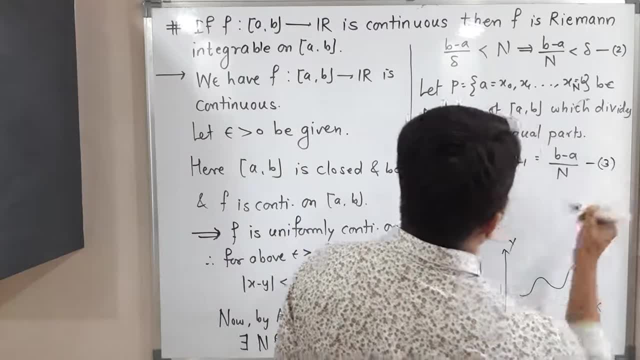 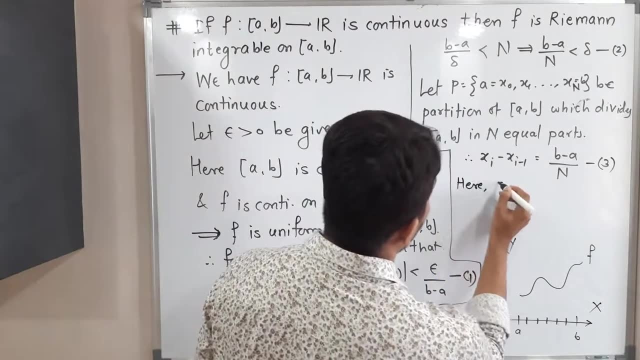 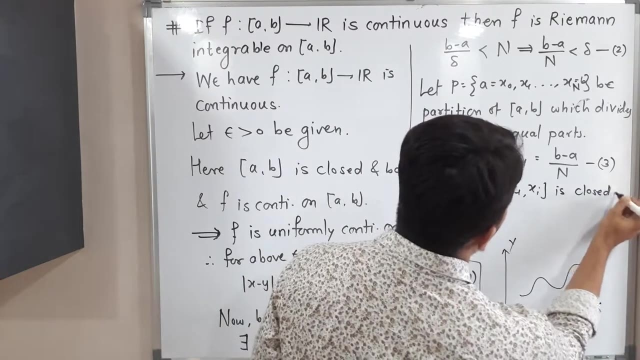 So this is also very important thing- I will call it as 3.. So let us continue What we have here. I am talking about a subinterval. xi minus 1. xi is close and bounded okay, So obviously it is a close set. 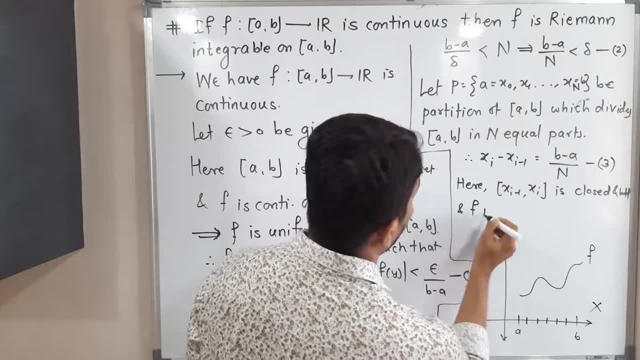 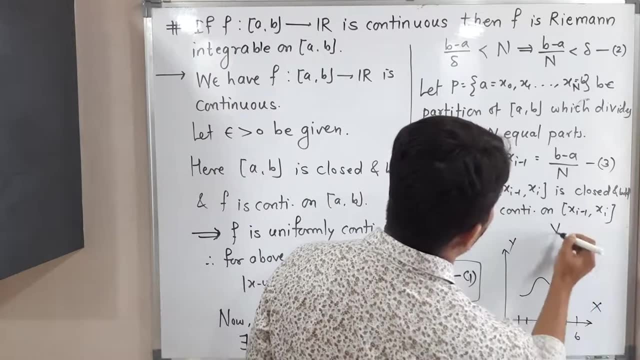 So it is close and bounded And f is continuous on xi minus 1 xi. This is true for all i running from 1 to n. okay, So, very important thing, I am writing. So if you consider any subinterval, okay. 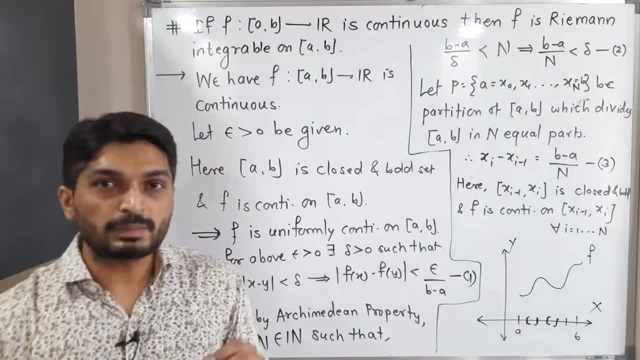 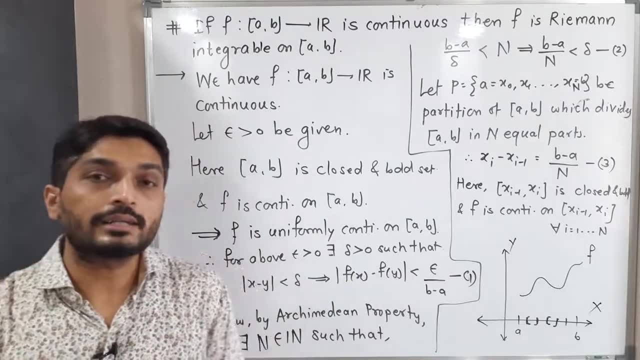 This one or this one, anyone okay? So function is basically continuous on close interval AB, So it is continuous on that subinterval also. So there is one more result. That result says function is also bounded and it attends its bound. okay. 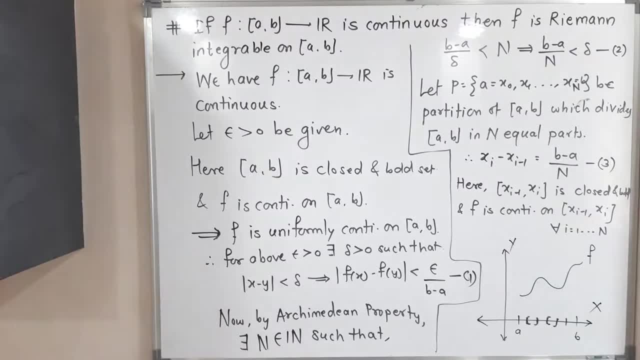 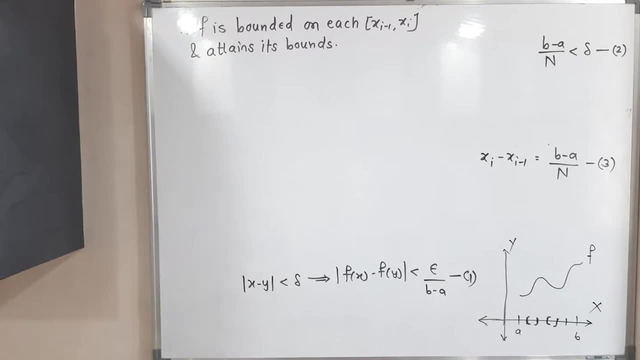 So that is a very important thing, But see, there is no more space to write. Make a screenshot of it, Okay. Okay, Then we will go further. So important equations are kept as it is. okay. So we have reached up to this. 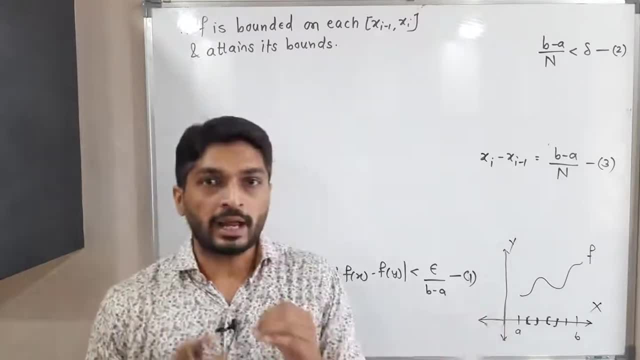 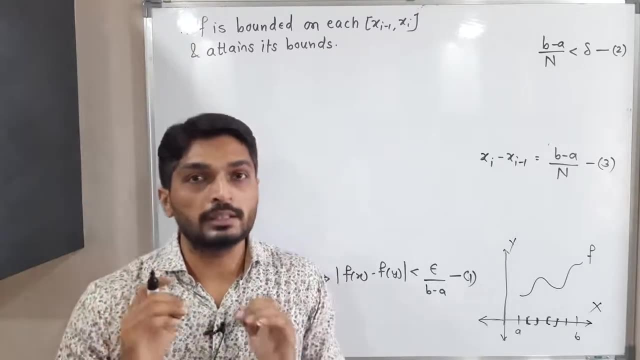 So function is bounded on each subinterval and attends its bound. That means there is one point where function will have the maximum value And again there is one point where the function has a minimum value. So after that I will consider capital, MI, small mi. 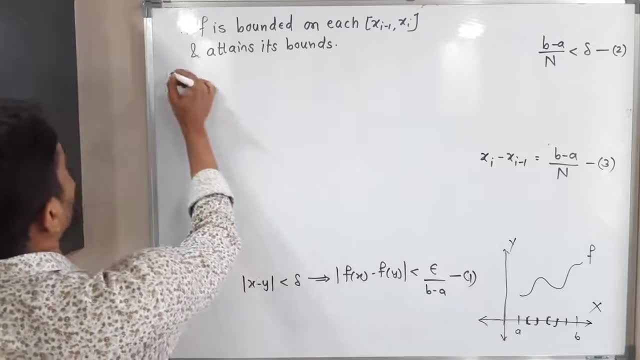 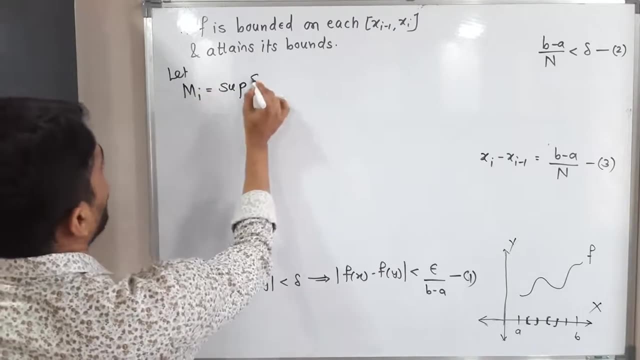 You are already familiar with definition, So let me write: okay, So let capital MI. you know the capital MI means supremum. Okay, let me write here: supremum of f of x, such that xi minus 1, less than or equal to x, less than or equal to xi. 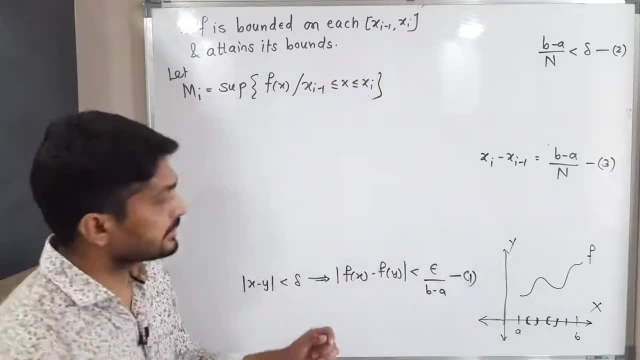 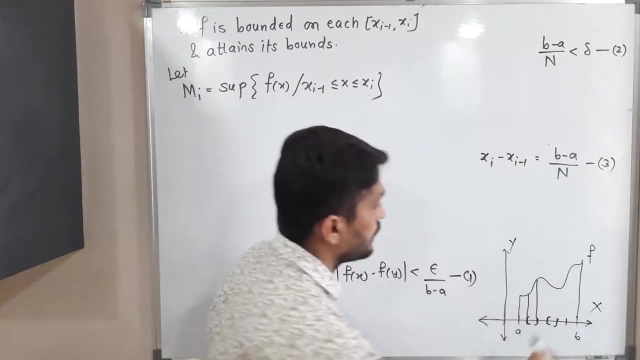 Okay, xi. So see, yes, this is that means in each subinterval, function will have some maximum value and some minimum value. In this way you can continue. So function will have some maximum value, that is capital MI in each subinterval. 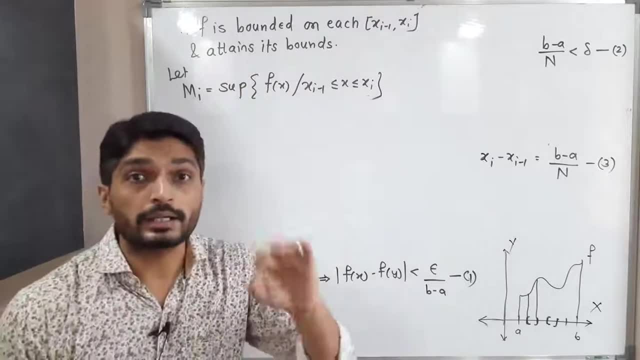 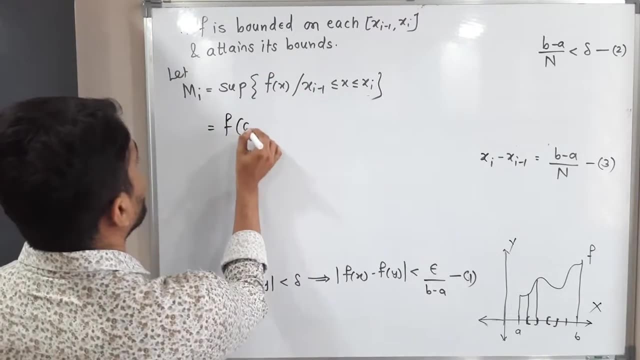 And, as I mentioned here, it attends its bound. attends its bound. That means there is one point Where the function has a maximum value. So you can consider that is f of ai. Again, it is true for all i running from 1 to n. 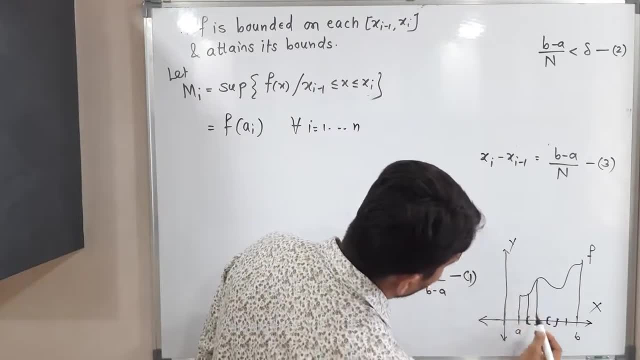 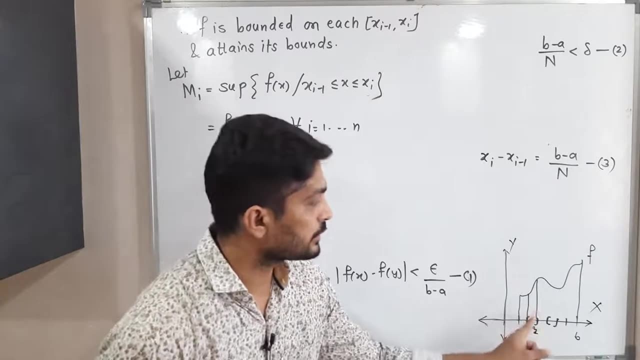 So what I want to say. So, as you know, here the function has a maximum value here. So there will be some here: ai or a2, if you consider the second interval In second interval, function has a maximum value at this point, at this point. 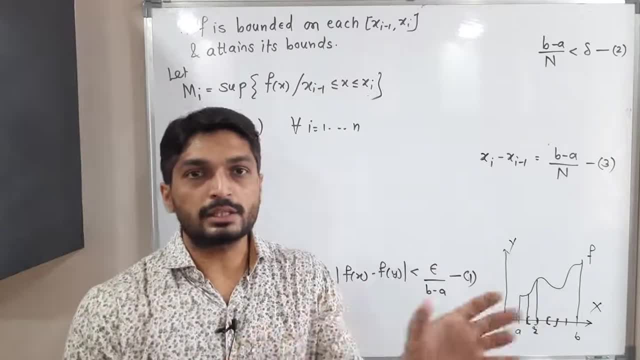 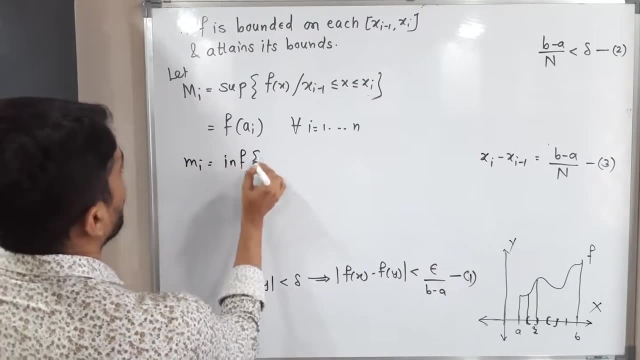 So that point will be a2 here. In this way, for each subinterval you will have the different different points. Let us go further. I will talk about small mi. You are familiar with it. Infimum of f of x, such that xi minus 1, less than or equal to x, less than or equal to xi. 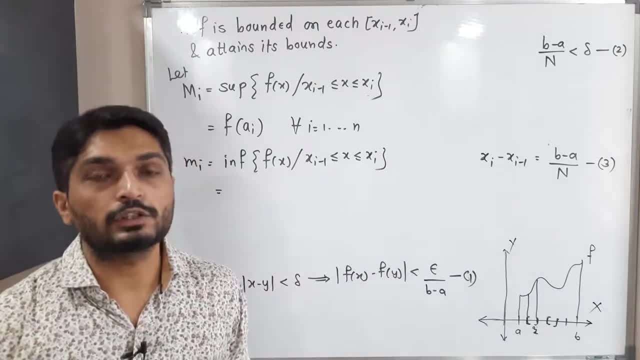 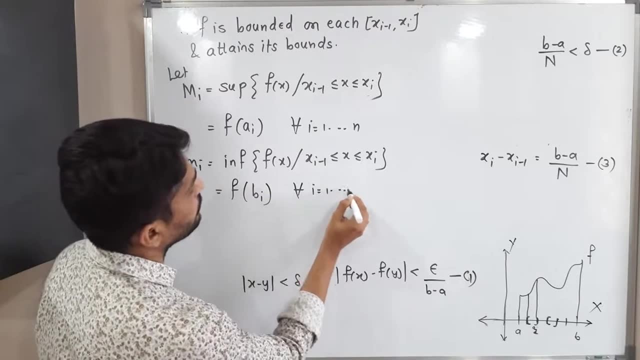 Again, the function attends its bound. That means there is one point where the function has a minimum value, So I will call it as bi. So f of bi you will have for all i running from 1 to n. Okay, 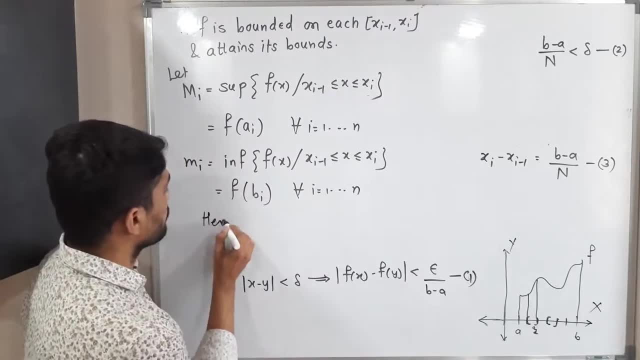 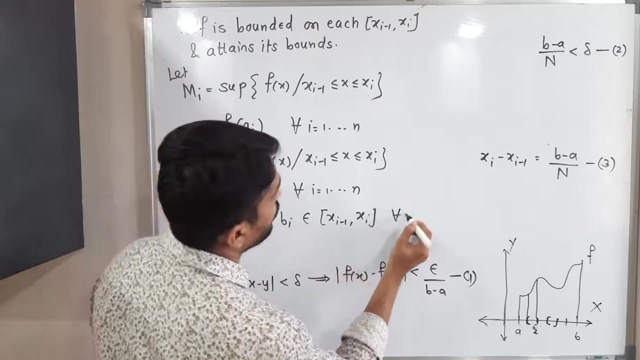 But see basically here. here I should mention ai and bi. Both of them are members of xi minus 1.. This is true for all i running from 1 to n. That means for first subinterval you will have some a1, b1. 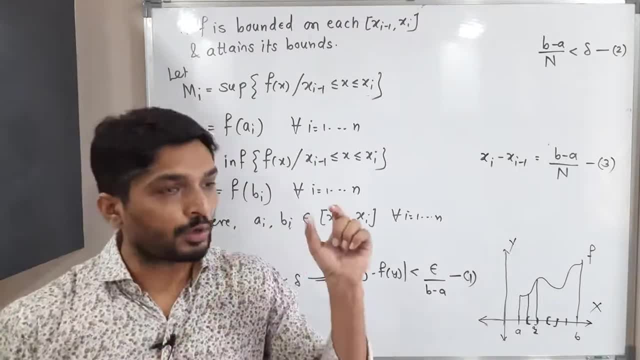 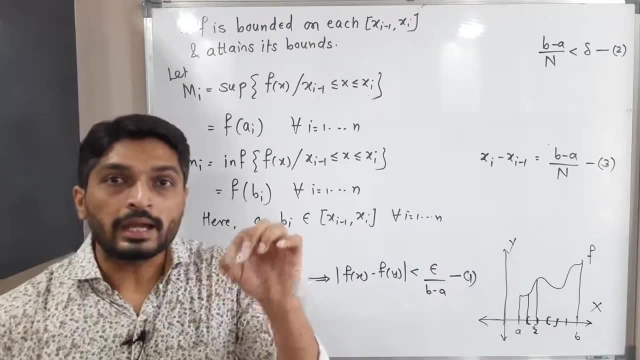 For second subinterval, you will have some a2, b2.. For third subinterval, you will have some a3, b3.. In this way, in each subinterval you will, you will find this ai and bi. Ai, that means a point where the function has a maximum value. 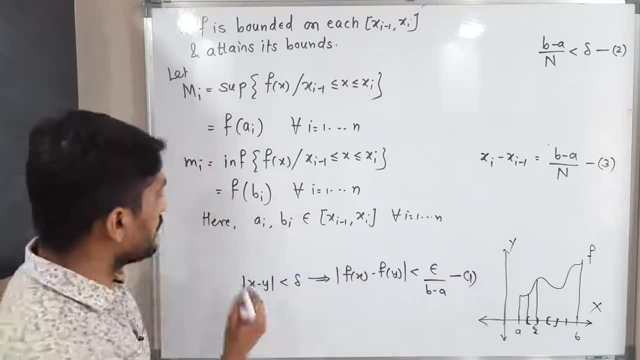 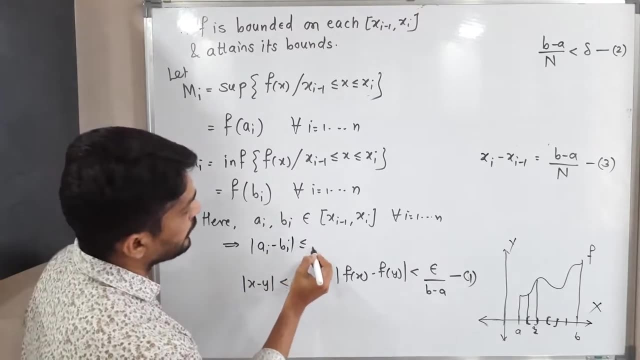 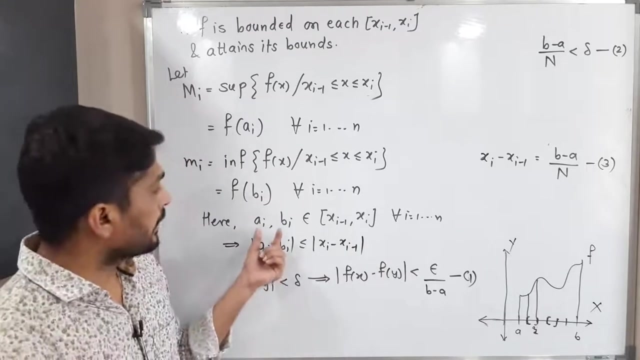 And bi means a point where the function has minimum value. So therefore, therefore, mod ai minus bi. Okay, Mod ai minus bi less than or equal to mod xi minus xi minus 1.. We are getting see ai bi, for example, if you consider this subinterval. 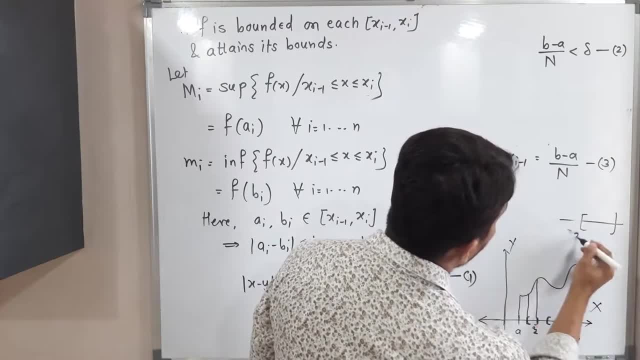 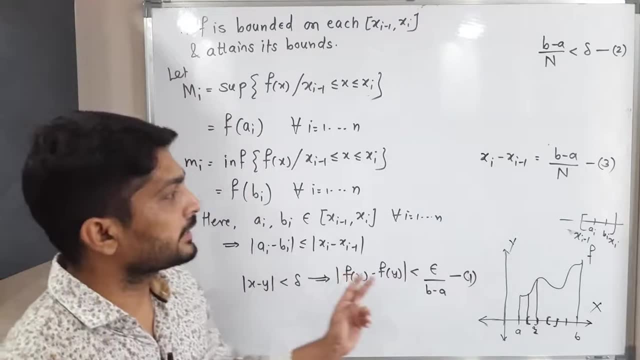 Okay, I am considering: like this is a, this is xi minus 1 and this is xi, Here is some ai, Here is some bi. Getting So mod ai minus bi, that means distance between ai and bi is less than or equal to length of that interval. 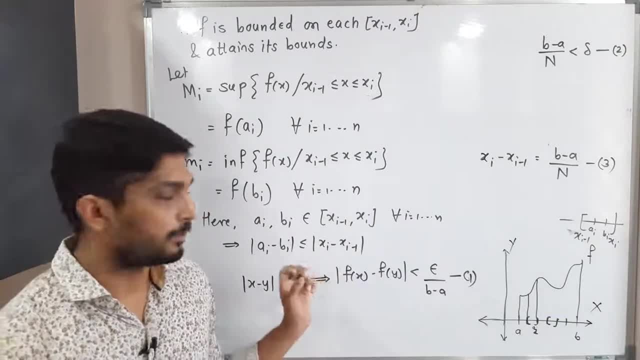 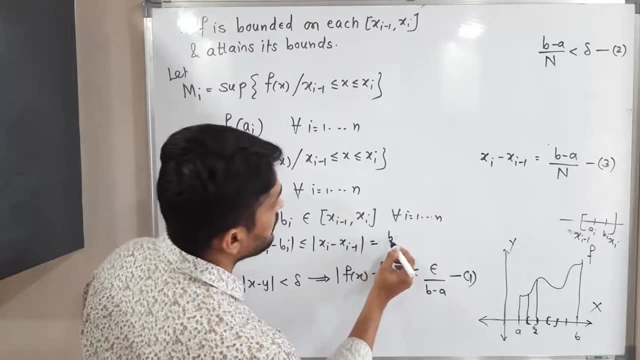 xi minus xi. So xi minus xi minus 1 means length of that interval. This thing we have, Okay. So xi minus xi minus 1, we have seen it somewhere, Yes there. So its value will be b minus a by n. 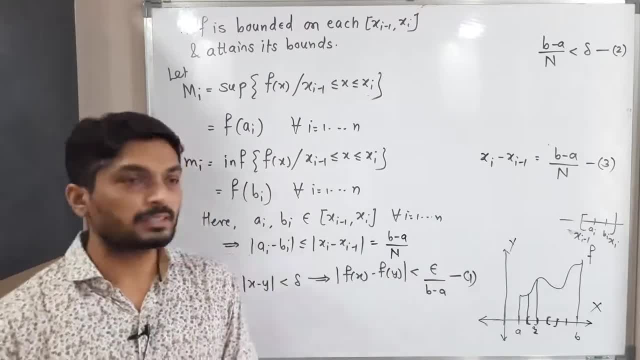 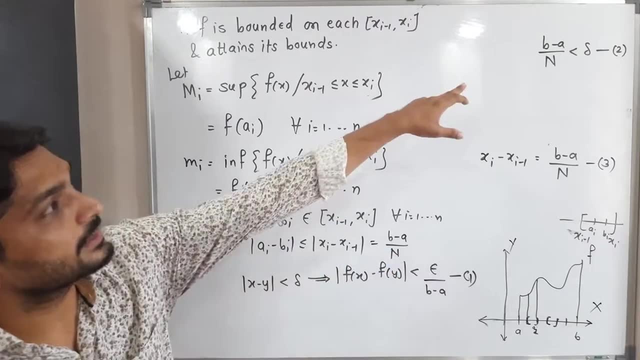 Actually no need to write mod, since it is a positive real number. So that is why I did not write mod here. See b minus a by n. we have seen it somewhere. That is inequality number 2. So it is less than delta. 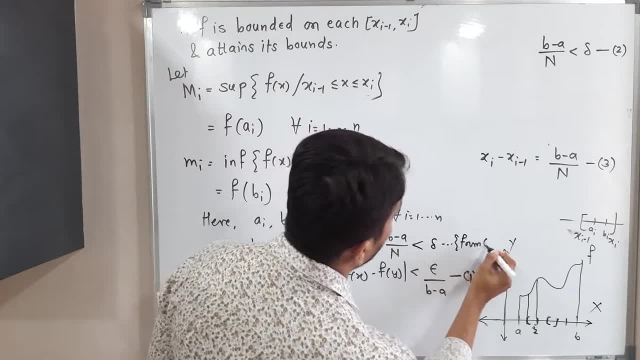 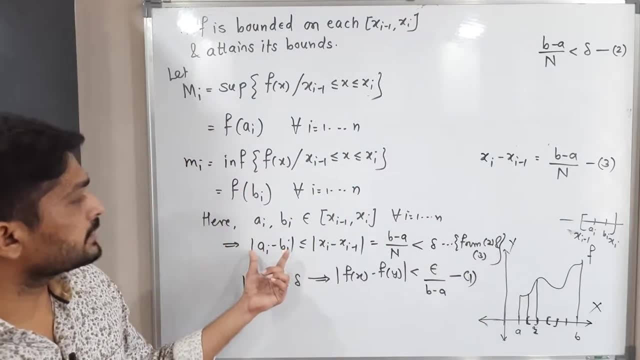 Okay, I should mention from: we use 2 and 3.. 2. And 3. So we use 2 and 3.. So see what it means. Mod ai minus bi less than delta. So can we use this statement number 1?? 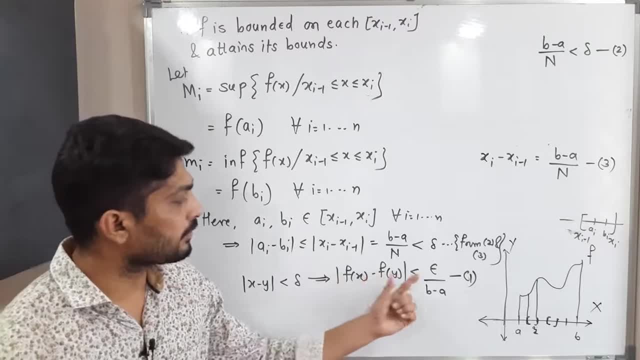 If mod x minus y less than delta, then mod f of x minus f of y less than epsilon by b minus a. So we can use 1 here. Okay, So I am going to use 1, but let me remove it 1.. 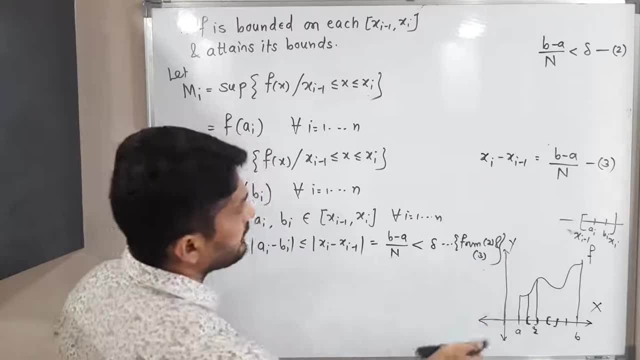 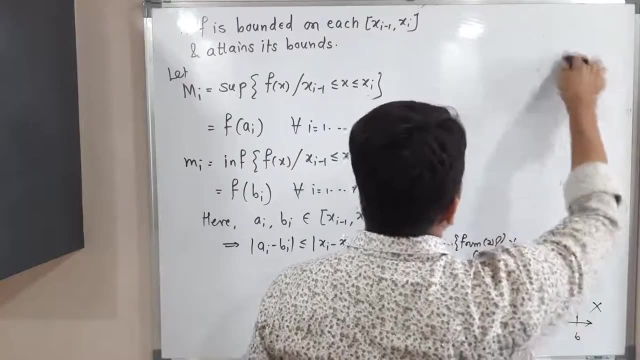 So we will have space to write Okay. So, yes, I will remove this one also. It is not required. now. We have used all these inequalities, Okay, And you have also Already made screenshots of it. Okay, Let us go further. 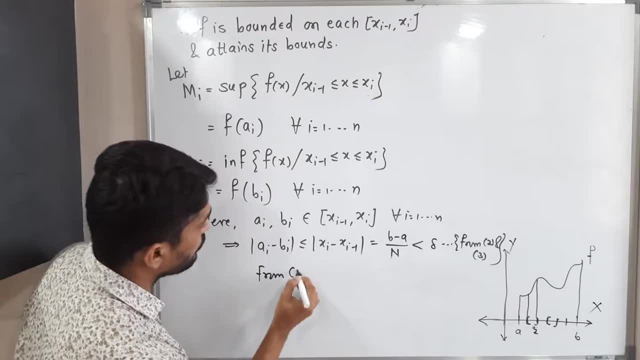 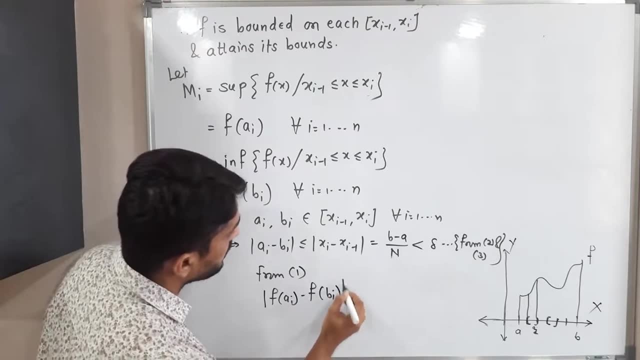 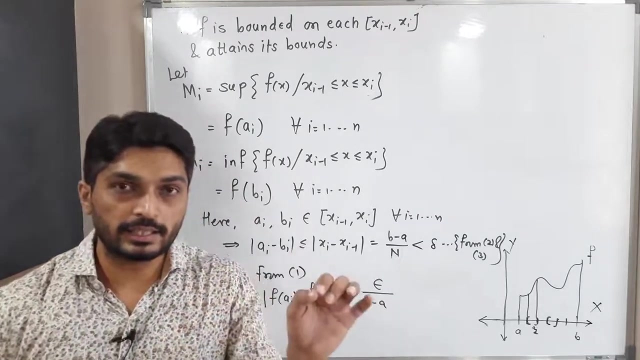 So yes, From 1, now From 1.. What will we have From 1.. Mod f of ai minus f of bi less than epsilon by b minus a. From 1 directly we can write: Since 1 says mod x minus y less than delta implies mod f of x minus f of y less than epsilon by b minus a. 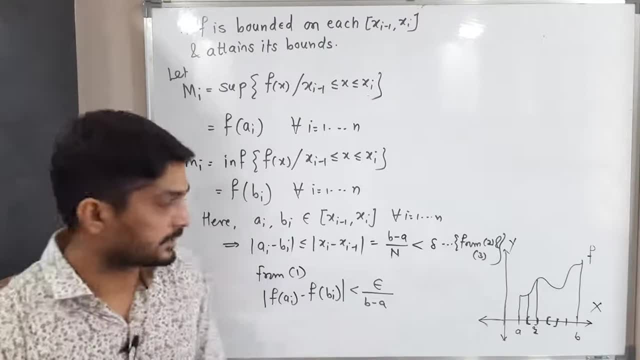 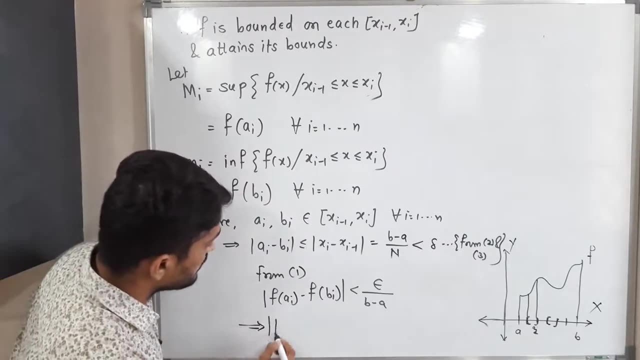 So, at a place of x and y, simply we have ai and bi. This is the only difference, See. but f of ai? Have you seen it anywhere? Yes, It is nothing but capital mi. So we can say: this is capital mi. 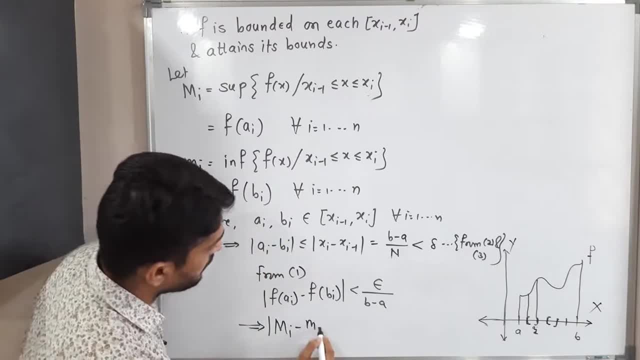 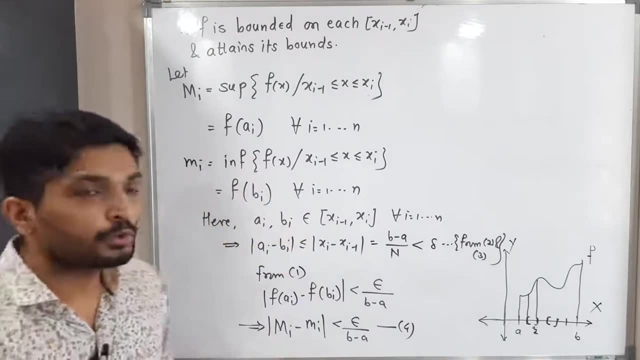 f of bi, that is nothing but small mi. Small mi less than epsilon by b minus a. This is called it as 4. Getting. Actually, there is no need of mod, since capital m is obviously greater than or equal to small mi. 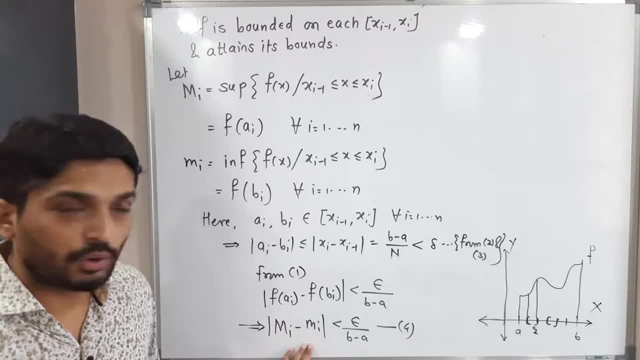 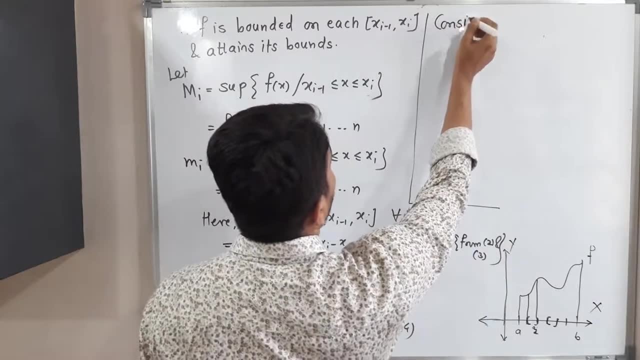 So it will have a positive value getting. So no need to write mod, You can write as it is. Let us go further. Okay, So now what I am going to do? Consider. I am going to consider upf minus lpf. 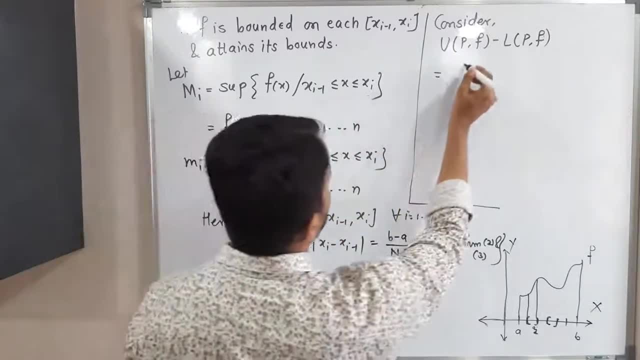 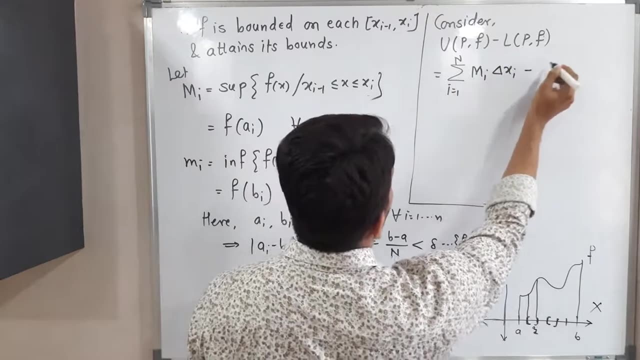 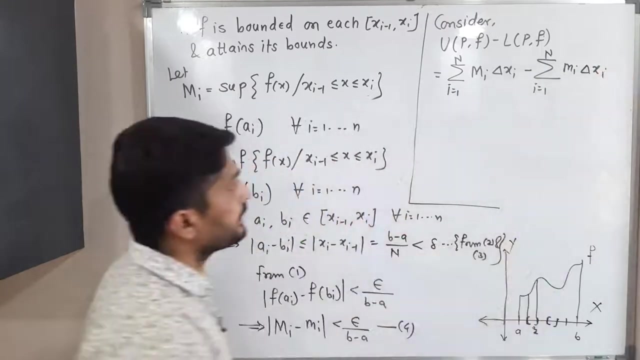 What is upf? You remember? Upf means summation, A person, we call it as I. running from 1 to n- Capital, mi delta xi. minus summation. i. running from 1 to n- Small, mi delta xi. What can we take common? 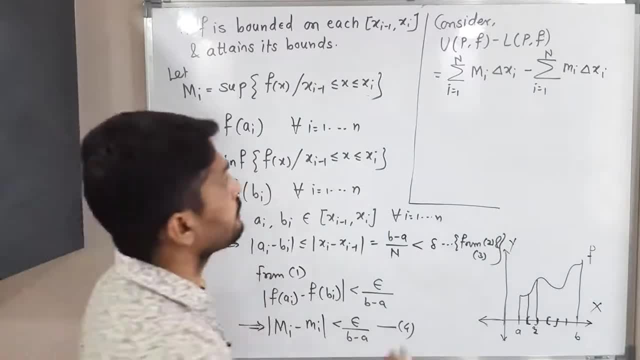 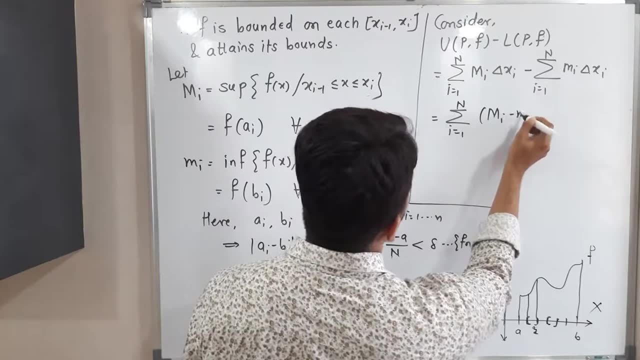 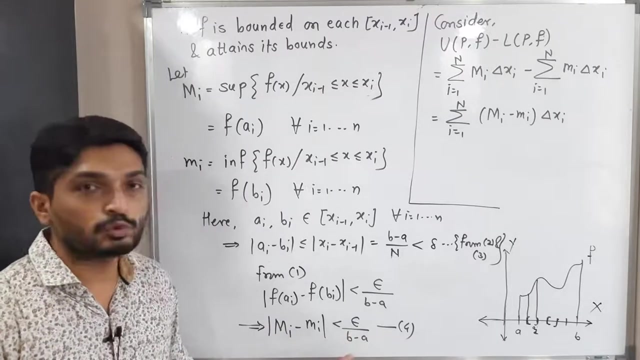 We can take summation common. We can take delta xi common. So obviously we can write: this is equal to summation common. I have taken right and capital mi minus small mi, delta xi. But as we have got here capital mi minus small mi less than epsilon by b minus a. 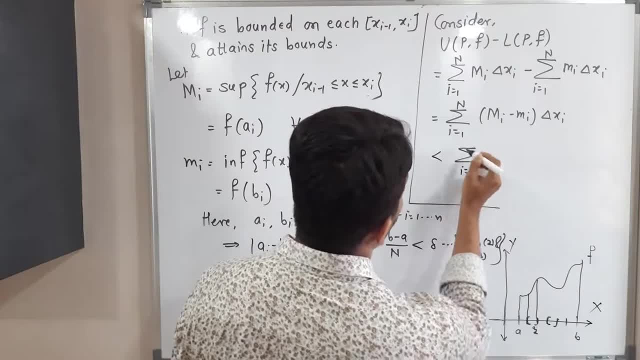 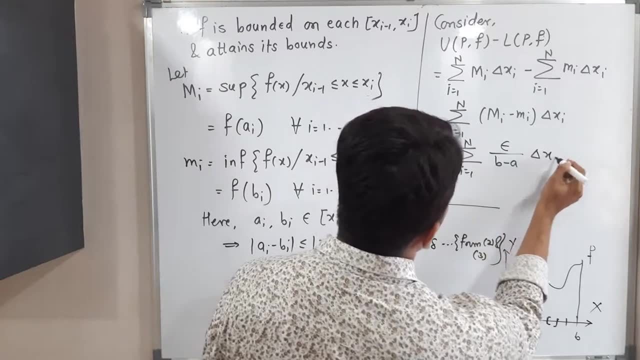 So let me mention this is less than summation. I running from 1 to n, Epsilon by. let me write epsilon by: b minus a, delta xi. Okay, So yes, there is no more space. So let me remove this diagram and then we will continue. 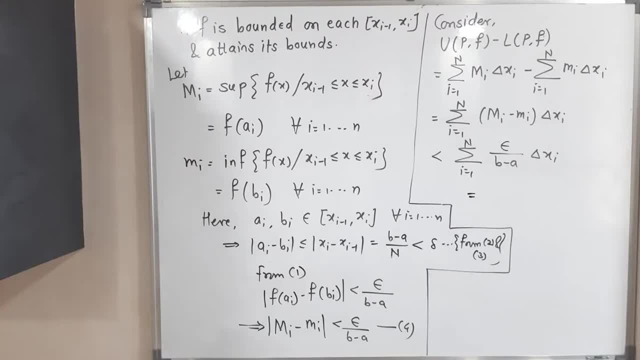 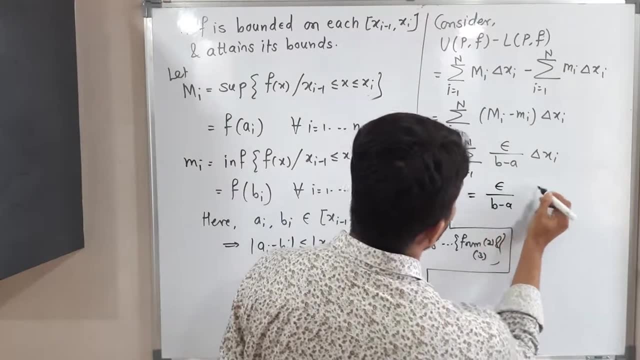 Okay, Let us continue now. So epsilon upon b minus a is independent. on that i summation getting, So we can take it outside. So epsilon by b minus a, So summation i running from 1 to n: delta xi capital. 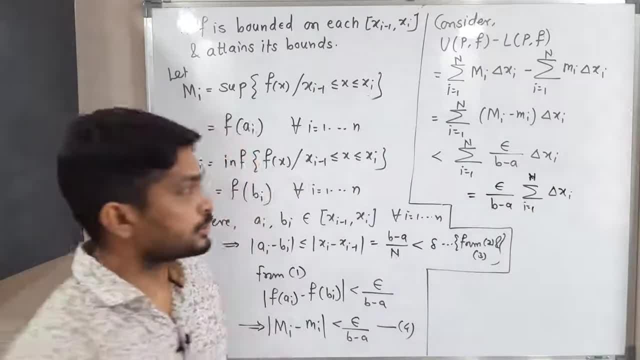 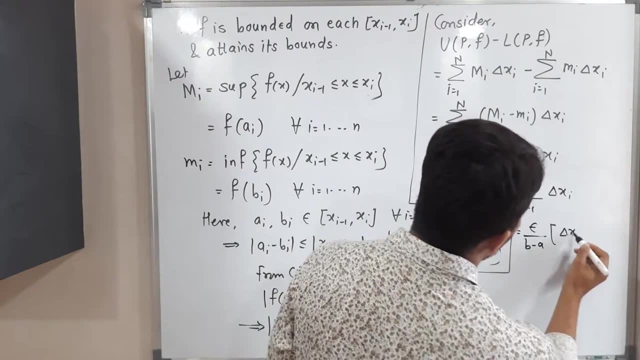 Okay, So see what will I do. I will expand the summation So we will have: Okay, Let me write it. Yes, So this is equal to epsilon by b minus a. If I put i, So i is equal to 1 delta x1.. 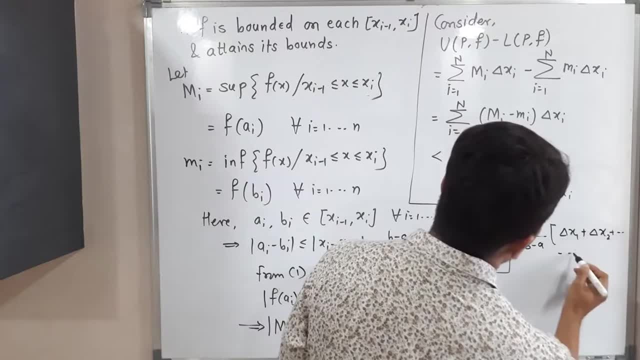 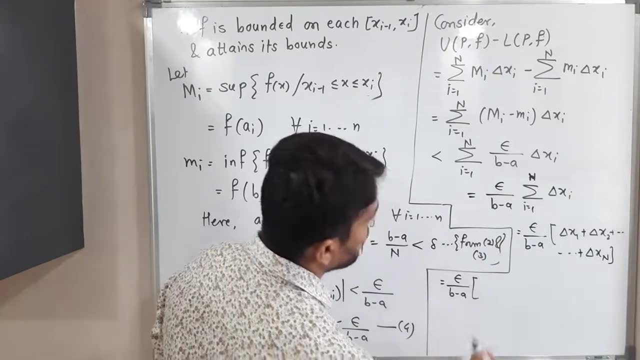 If you have put i is equal to 2, delta x2 plus and so on, We will have delta xn. Let us put the values So this is equal to epsilon by b minus a. Delta x1 means x1 minus x0. 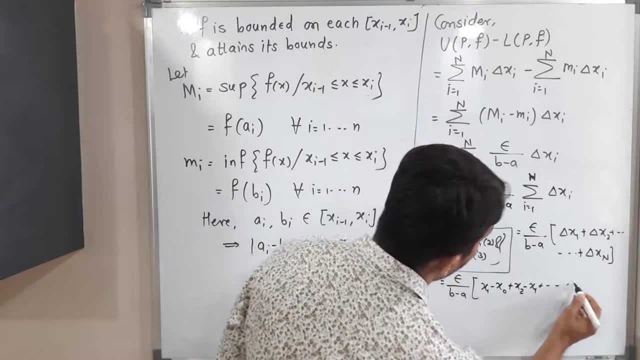 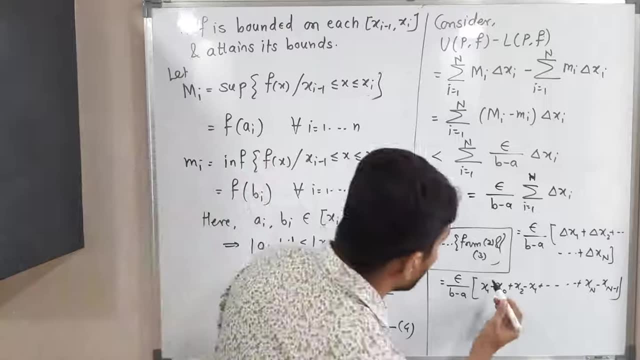 Delta x2 means x2 minus x1, and so on. Delta xn means xn minus xn minus 1.. So what will happen? All terms will get cancelled, Just like this x1 minus x1.. This x2 minus x2 will get cancelled. 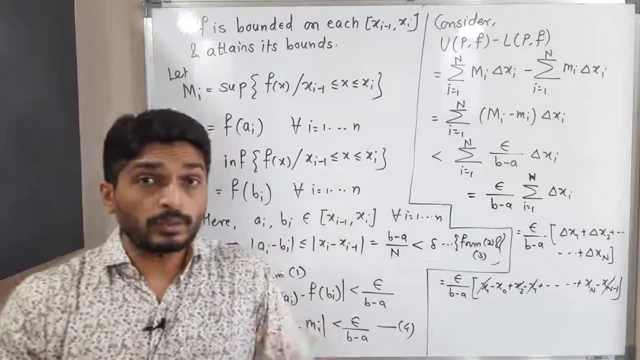 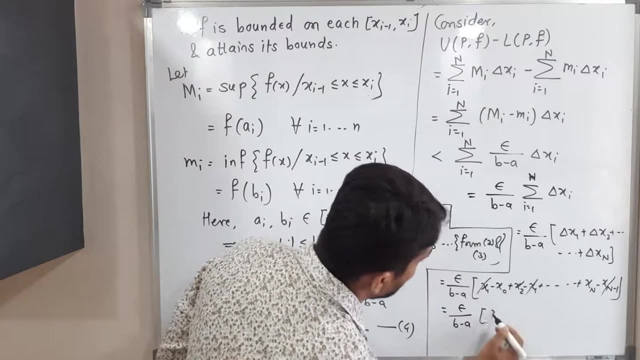 And this minus xn also And minus 1 also will get cancelled. Only first and last terms will be there. So this is equal to epsilon by b minus a. Last term means xn, First term means x0. So you know that x0. 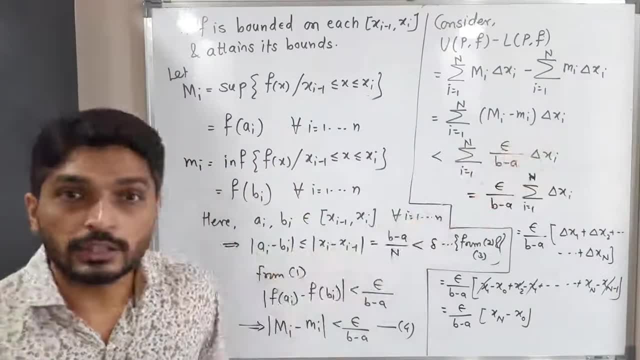 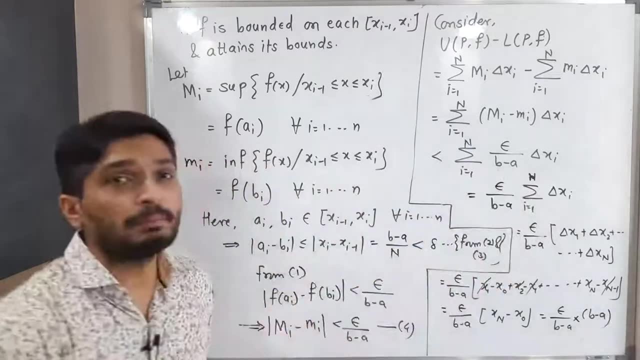 First term, That is nothing but a, Xn. Last term, which is nothing but b. So this is equal to epsilon by b minus a into b minus a. So I am so much happy to cancel that b minus a, b minus a, b minus a cancel. 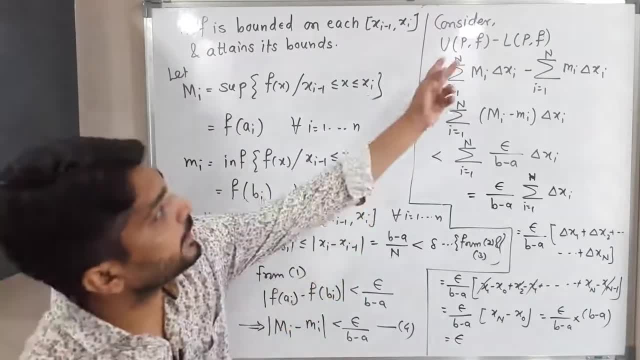 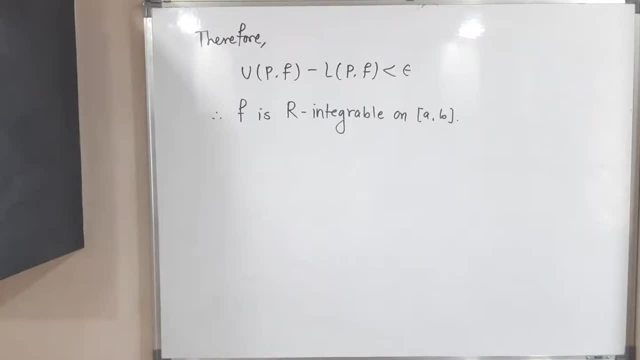 We will have epsilon. So, finally, what can we say? We started with Upper sum minus lower sum And we got it is less than epsilon. Okay, So, in short, we can write UPF minus LPF, less than epsilon.